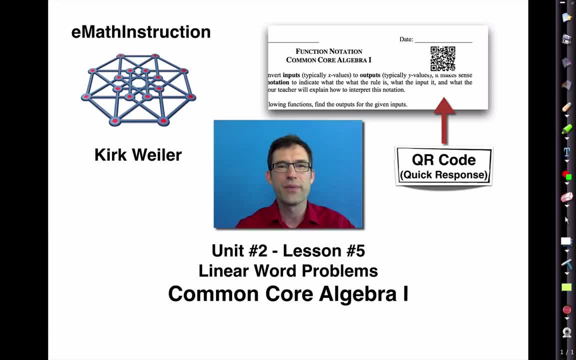 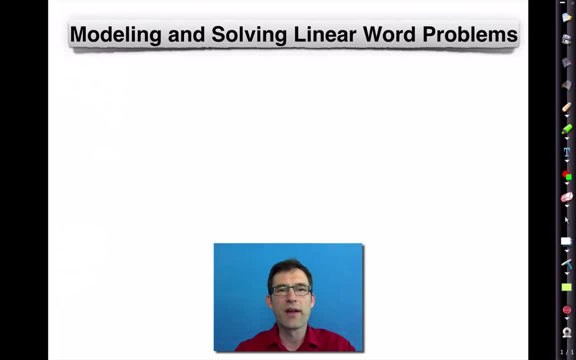 You know you love them, You know you're excited about them. Let's do them. So modeling and solving linear word problems: It's hard to really give a recipe or anything like that for this, so take these sort of bulleted points more as pieces of advice, things that are good habits of mine, that 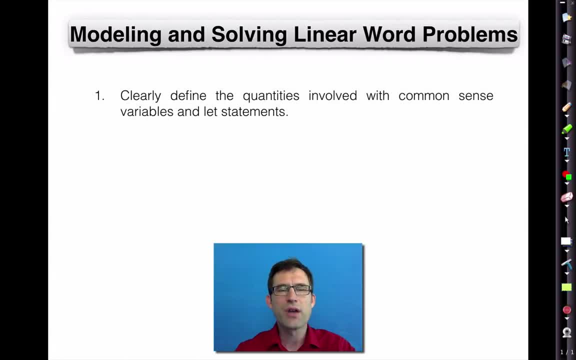 will help you. So let's get started. So first, you always want to clearly define the quantities involved with common sense variables and let statements. Choose good letters, letters that make sense to you. Do really good let statements so that you have no doubt about what things you're actually representing with the 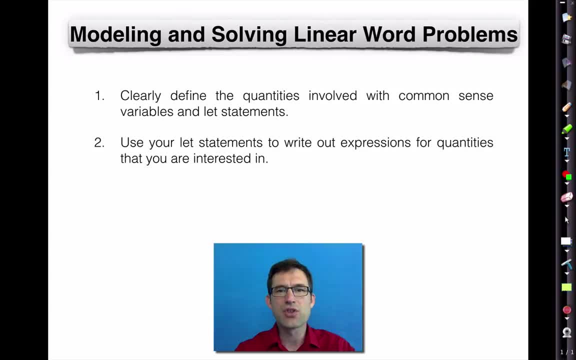 variables. Number two, use your let statements to write out expressions for quantities that you're interested in. In other words, when we did that translation lesson a couple lessons ago, we did that translation lesson, We did that translation lesson. We did that translation lesson. 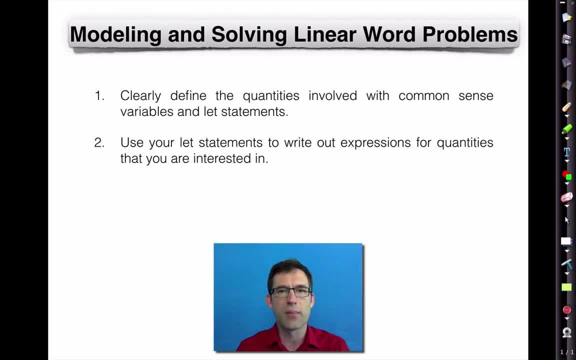 where we were translating English into math. That's step number two. You want to be very careful to write out expressions that you're interested in using those. let statements Number three carefully translate the information that you're told in the problem into an equation, right? 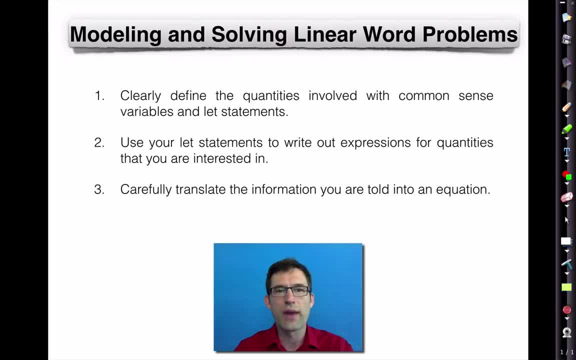 Ultimately, there's going to be information that allows you to write an equation that you can then solve. Solve that equation, though, and, just like we did in the last lesson, make sure that you're mentally just happy with what you're doing. So let's get started. 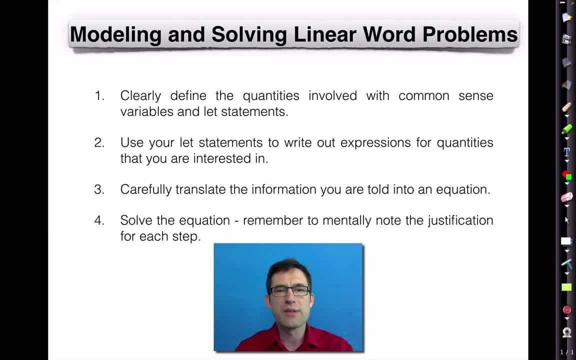 First, you're going to be justifying every step. Eventually, of course, you're going to be solving equations almost by rote. You know, you just get into it to a point where you're not thinking about the justifications, But right now it's important to be thinking. I just used the commutative. 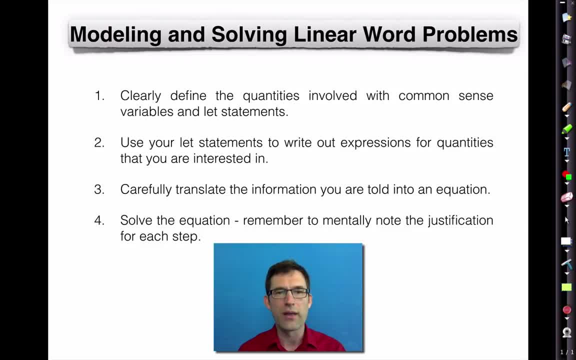 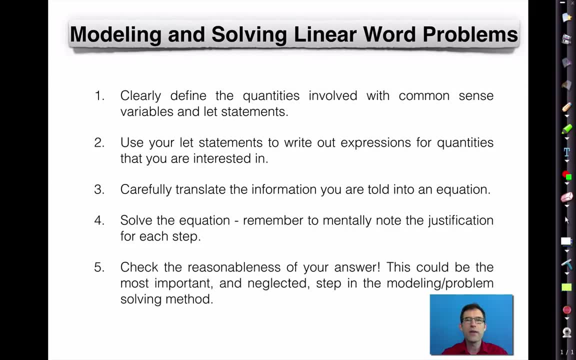 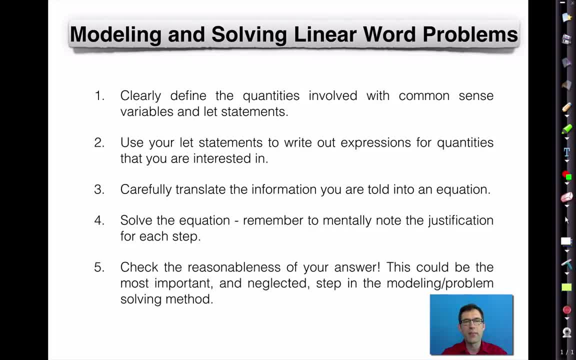 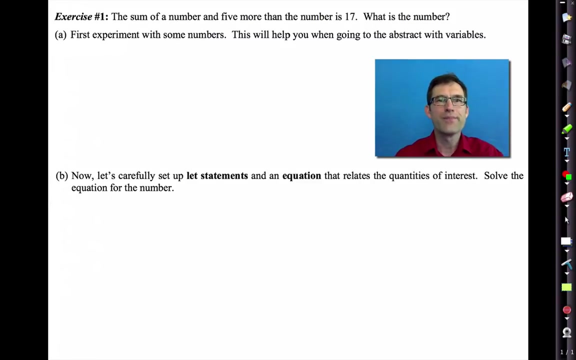 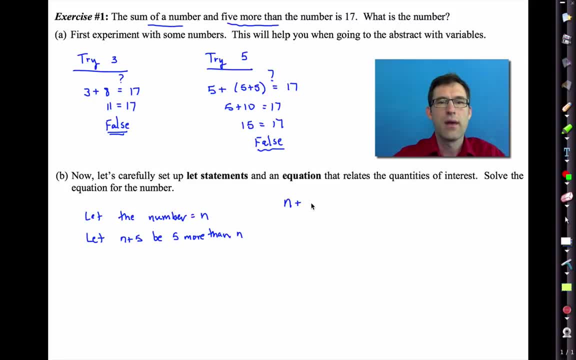 So we're going to sum, right. We're going to sum n and n plus 5, and that's going to be 17.. Now a lot of people wonder why I put the n plus 5 in parentheses. Number one: it's safe. 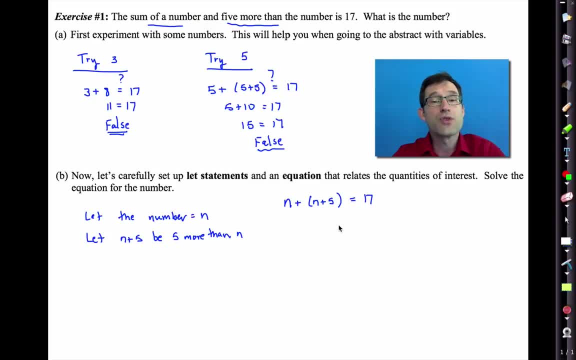 But number two. it's correct. In other words, the two numbers are n and n plus 5, right? So n plus 5 is its own thing, It's its own quantity. But now I'm going to use some properties to solve this equation, right? For instance, 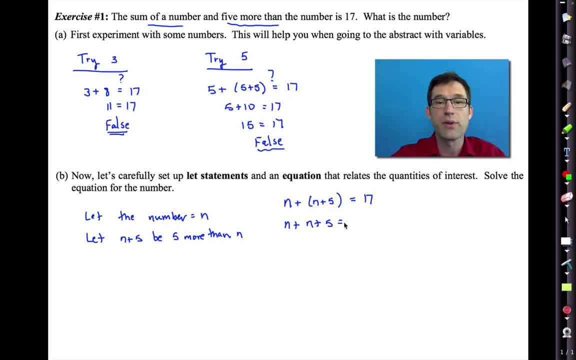 I'm going to use the associative property of addition to simply remove the parentheses, Because I know that when I add three things together, I can add any two of them I want. So, in other words, I'm going to actually add these two n's first, before I add the. 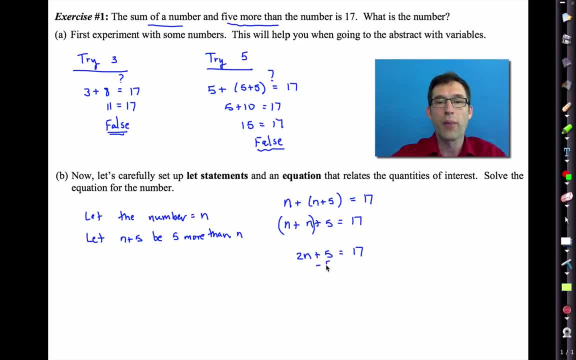 5.. Now I'm going to do a little additive property of equality right by adding negative 5 to both sides. That's going to leave me with a negative 5.. That's going to leave me with 2n equals 12.. 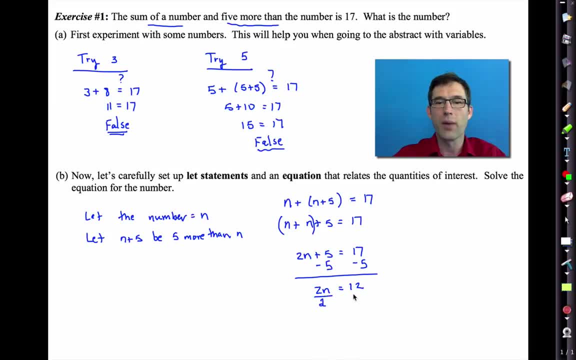 That almost looks like Zn. Then I'm going to use the multiplicative property of equality to multiply both sides by 1, half, or divide both sides by 2. So I find out that the number is 6.. Now of course I can check this pretty easily, because this one at least I can take my number. 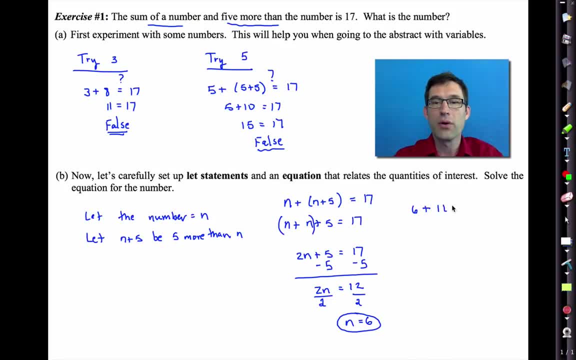 6,. I can add it to 5, more than the number which is 11. now that almost looks like a 12.. And I can find that the number is 6.. Now I know that that is, in fact, now a true statement, right. 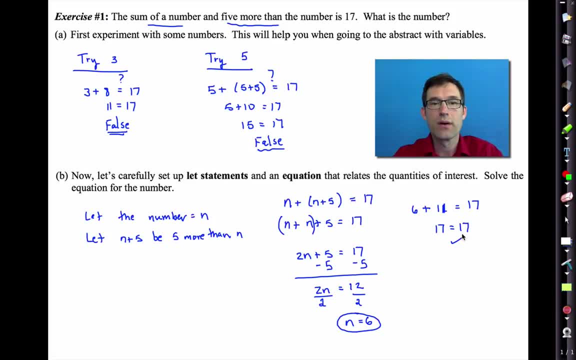 That actually makes the statement true. Okay, So careful let statements, careful translating of the let statements into an equation and then solving the equation using techniques we already know. Now, this one was pretty easy. we'll get into some more complicated ones in a bit, but take 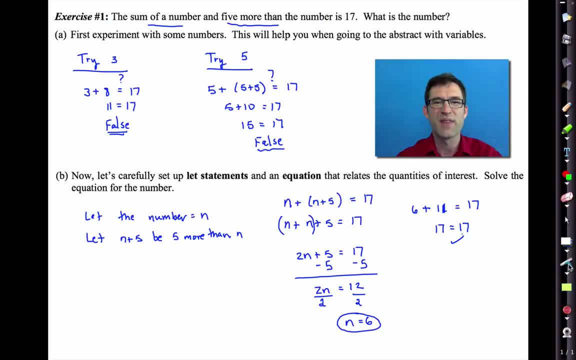 a look at that one, pause the video, write down anything you need and then we'll do some more. Alright, Now, ultimately, what we're always doing here is we're modeling. We're modeling a real world physical situation. Alright, maybe exercise one wasn't so much, but we will be, But we're. 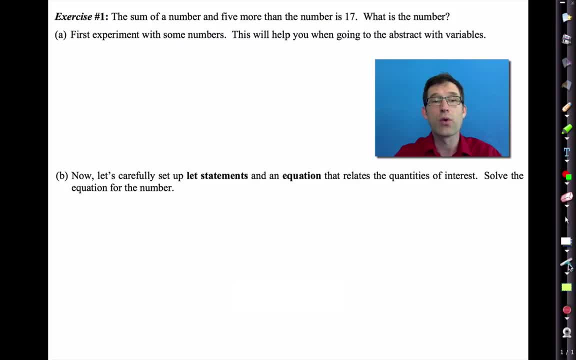 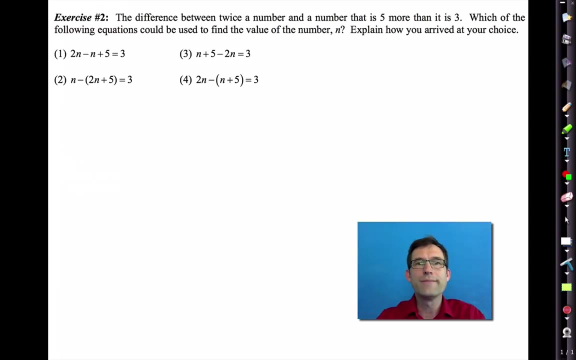 modeling it with equations, with symbols, and then we're allowing that modeling process to play out to give us the correct solutions. Alright, let's go on and look at the next problem. Alright, nice multiple choice problem. The difference between twice a number and a number. 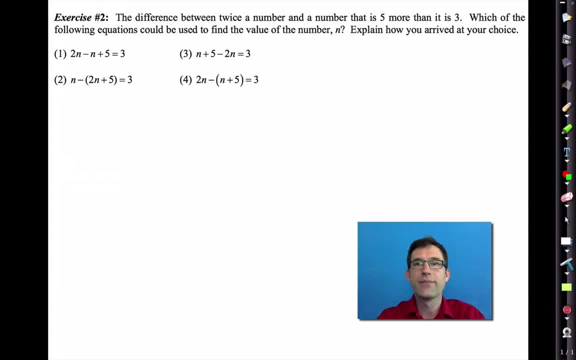 that is five more than it is three. Which of the following equations could be used to find the value of the number n? Explain how you arrived at your choice. So what I'd like you to do is pause the video right now and see if you can figure out which of the four multiple 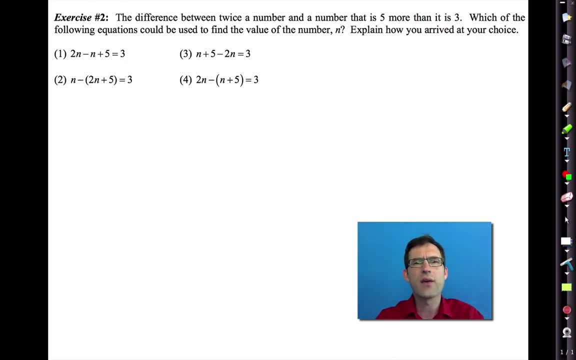 choice answers is the correct one and how you went about thinking about it. Alright, let's go through it. So the difference right. Difference means subtraction. Now we have to be careful with subtraction right, Because subtraction is not commutative. We have to make 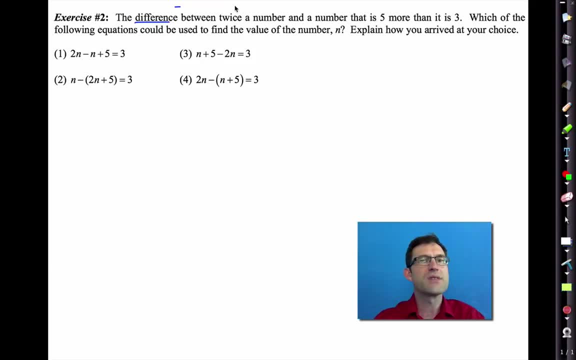 sure we do the subtraction in the right order. So they'll always give us the first number first, if you will. So the difference between twice a number. Well, if the number is n, then twice the number is 2n, right? 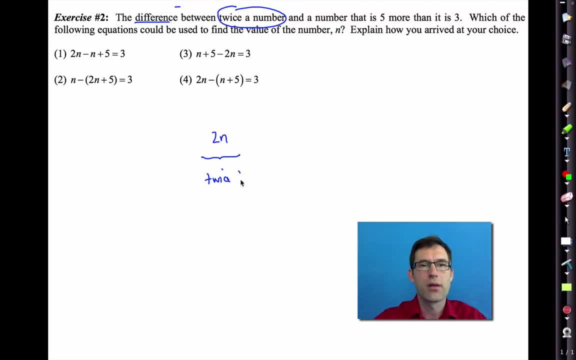 This is twice the number, Twice the number. That does not look at all like the word twice, It looks like twia, There we go. Twice the number, So the difference between twice the number and a number that is five more than it. So what's a number five more than it? 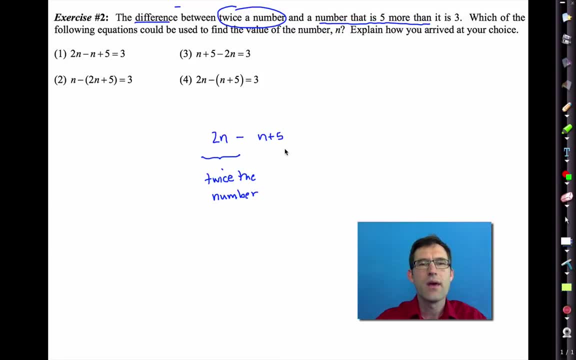 Well, n plus five, Right, And then it's equal to three. Now, if you put down choice one, well, that's a reasonable choice. The problem is it's wrong. And it's wrong because right now, what I'm doing is I'm doing 2n minus n, and then I'm adding five to the result. What I need to 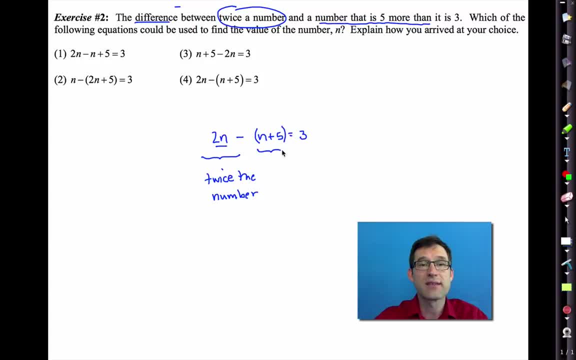 do is I need to do 2n minus a number, that is, five more, And because I'm subtracting the entire number, I have to have it in parentheses. All right, Maybe in the last problem having those parentheses around n plus five was somewhat irrelevant. I don't think it was, But maybe. 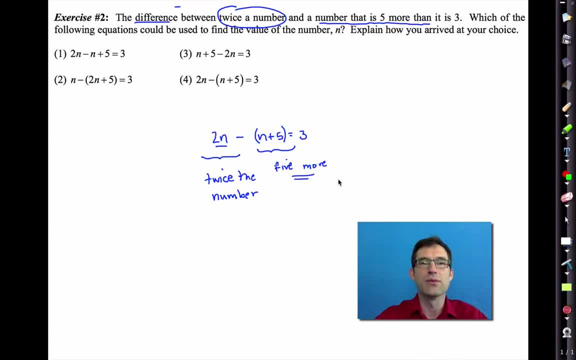 it was in terms of just solving the problem, But here it's absolutely critical because it's the difference between choice one and the correct choice, which is choice four. All right, I want you to think long and hard about that. Very important to have parentheses. 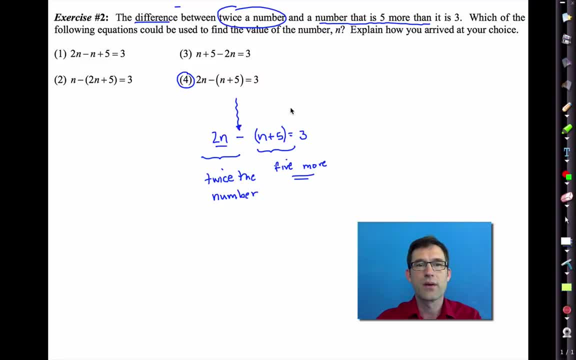 especially when you're dealing with subtraction. Okay, So I'm going to clear this out. Pause the video if you need to. I'm going to apparently move my arms around a lot. All right, Here we go, Let's move on. What can they throw? 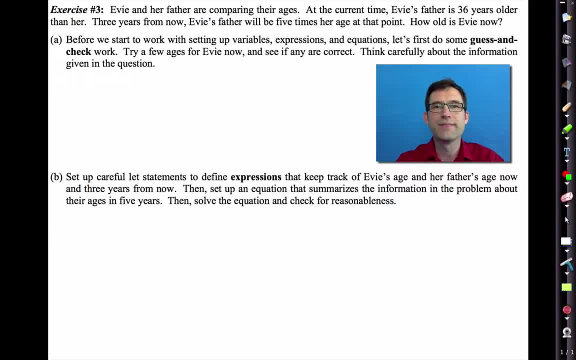 at me. Evie and her father are comparing their ages, All right. So Evie and her father are comparing their ages. At the current time, Evie's father is 36 years older than her. Three years from now, Evie's father will be five times her age. at that point, How old? 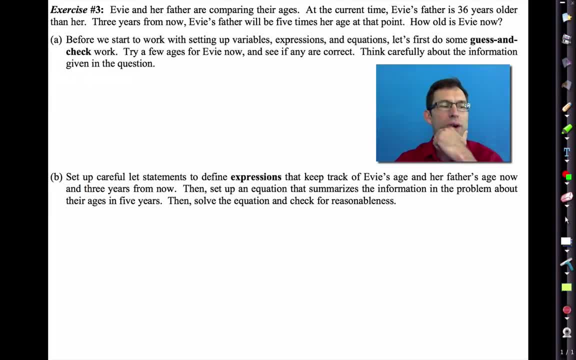 is Evie now? Whoo, All right. Well, why don't we try some guess and check? Okay, This is important. I often will tell students that it's a really, really good idea to do some guessing and checking before you launch into the algebra, because it'll help you All right. 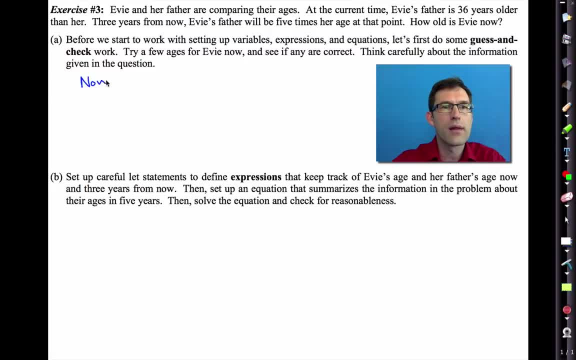 So let's do this, Let's keep track of their ages. Let's say that Evie is 10.. Okay, Then we're going to say dad instead of father, because it's a shorter word. What does it say? It says Evie's father is 36 years older than her. All right, So her dad will be 10 plus. 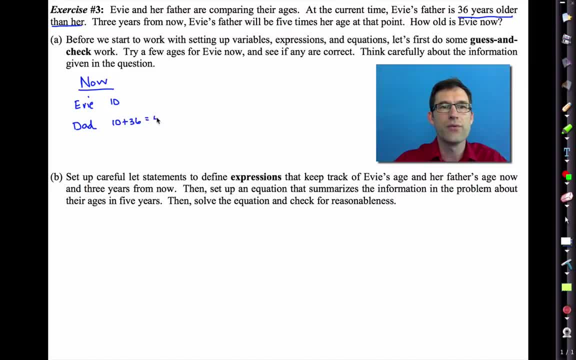 36.. All right, Which is obviously equal to 46.. All right, What is it? Three years older? All right. What is it Three years from now? Three years, Three years from now. Let's see what's going on. Well, three years from now, right, Evie will be 10 plus three. Now I 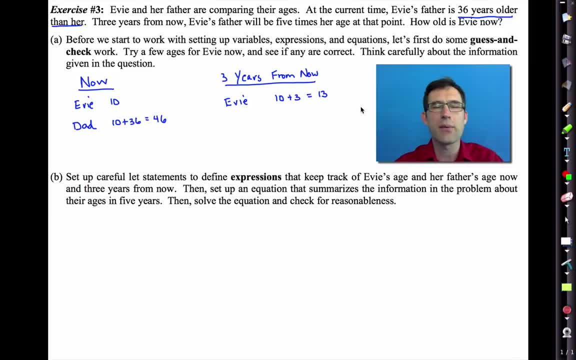 know that many of you would just write down thirteen, but again, I'm going to establish some algebraic background before we go on to Letter B. So Evie's going to be 13,, and And her dad would be well what? 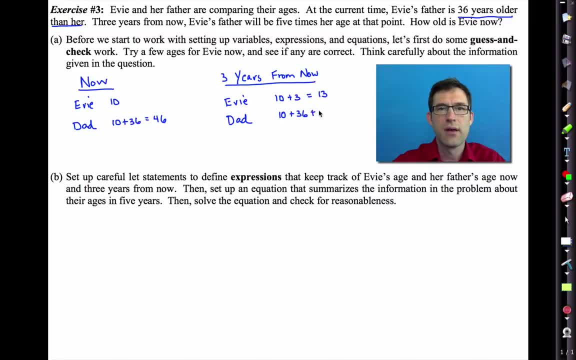 It would be 10 plus 36 plus 3, which would be 49. And it says Evie's father will be 5 times her age at that point. So the question was: were we right? Was Evie actually 10?? 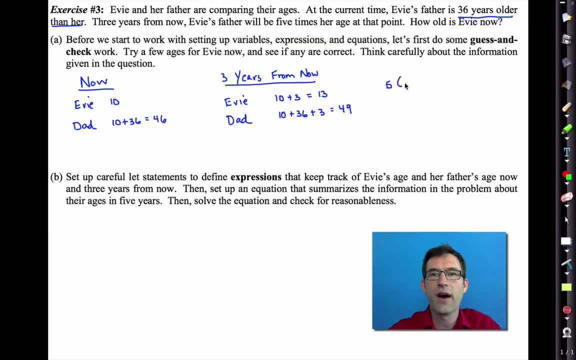 Well, we can check it by saying: well, is 5 times 13 equal to 49?? Right, Well, 5 times 13 is 65. And is 65 equal to 49?? No, that's false. So what does that really tell us? 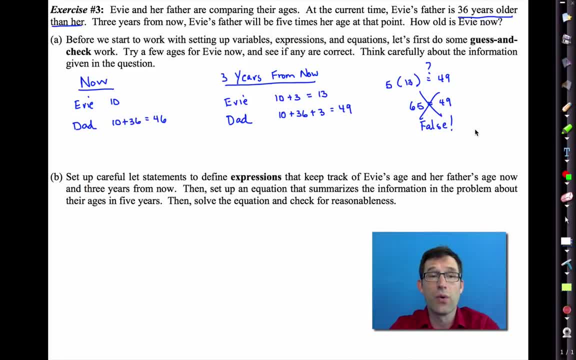 What it tells us is that Evie isn't 10 years old. All right, She just isn't. So let's now try to solve for Evie's age, All right. Now what we're going to do is we're going to essentially do exactly what we did before. 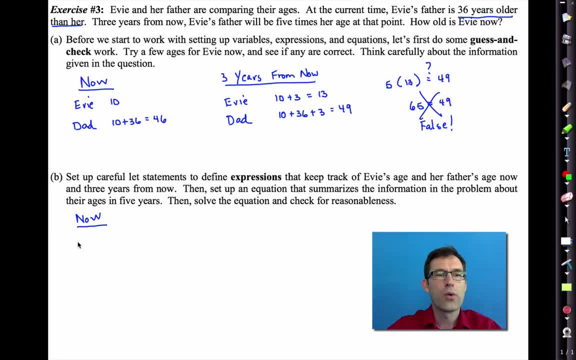 except instead of saying that Evie is 10,, we're going to let Evie's age be equal to. I don't like using E or A, I'm going to go with X. All right, If I don't like the variable that begins the word like E or A for age. 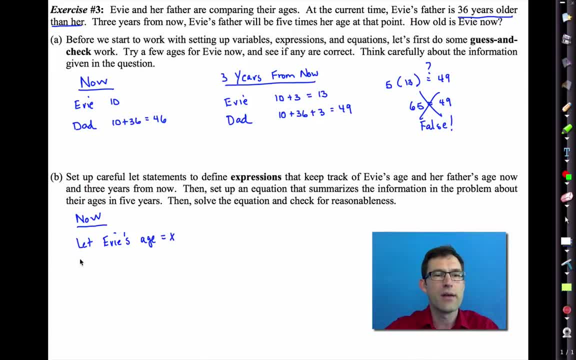 then I tend to go with X, X or Y. They're nice letters, Okay. So what's her dad? Well, her dad's age, dad's age. he's going to be 36 years older than her, So X plus 36.. 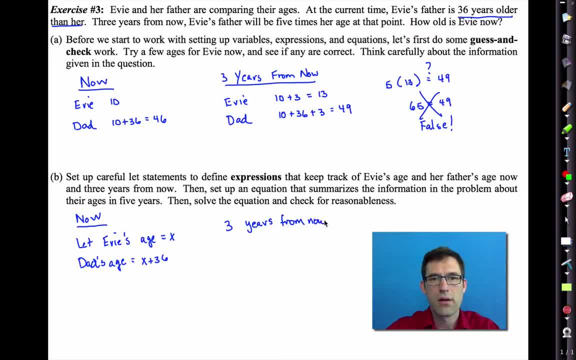 So, three years from now, what do we have? Well, three years from now, obviously, Evie's age is going to be X plus 3.. By the way, notice what I'm doing. Right, Everywhere that there was a 10, I'm basically now just putting in an X, right? 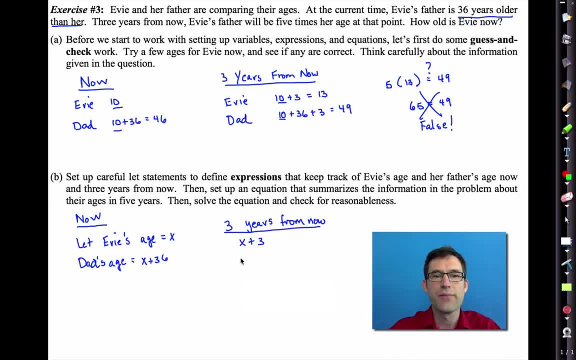 And watch me do that. So three years from now, Evie's going to be X plus 3, and Evie's dad is going to be X plus 36 plus 3, which is going to be X plus 39.. Now that final statement we're going to actually use to set up our equation, right? 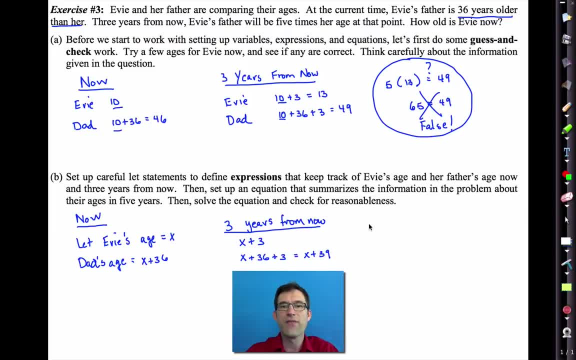 What we know is that Evie's dad is going to be X plus 36, right, Right, Right, Right, Right. So Evie's dad is going to be 5 times her age. So Evie's dad's age is X plus 39,. 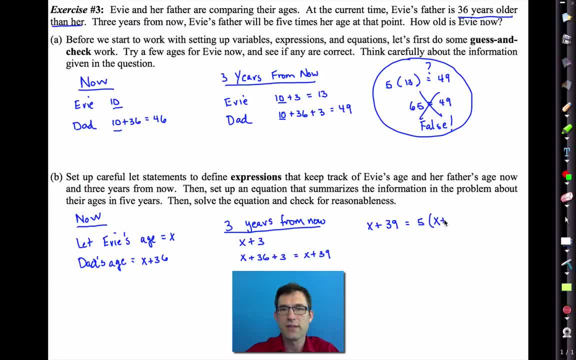 and Evie's age is 5 times X plus 3.. Now, please note, I kind of flip-flopped the order of the equation here. I kind of switched it a little bit, But we can now solve this right. 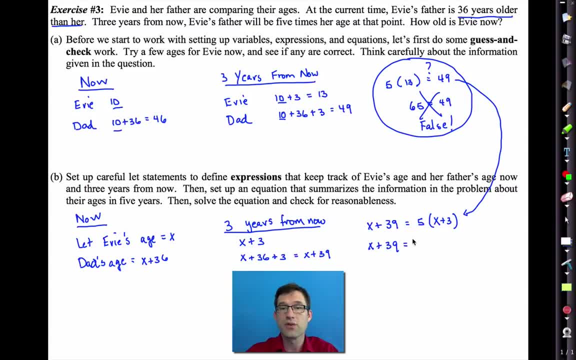 So X plus 39, I can now distribute, use the distributive property 5X plus 15.. I can now subtract an X from both sides using the additive property of equality, So I'll get: 39 is equal to 4X plus 15.. 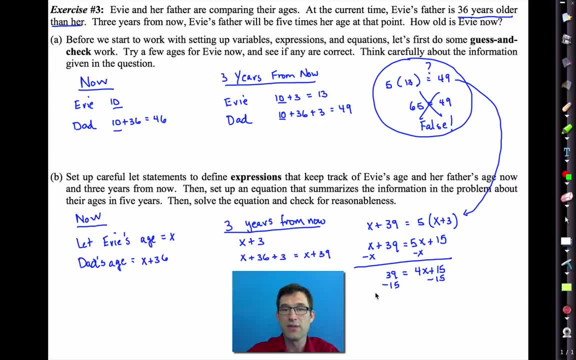 Likewise, I can subtract 15 from both sides, again using the additive property of equality, So I'll get: 24 is equal to 4X. And finally I'll divide both sides by 4 using the multiplicative property of equality. 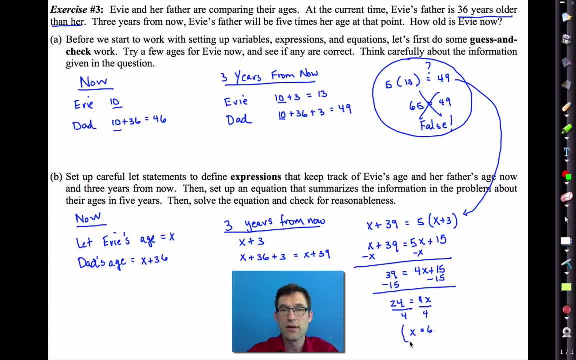 And I'll find out that Evie's age is 6.. All right, But notice how I was able to use what I did in Part A to walk myself through Part B. Whatever I was doing to the number that. I was sort of guessing and checking. 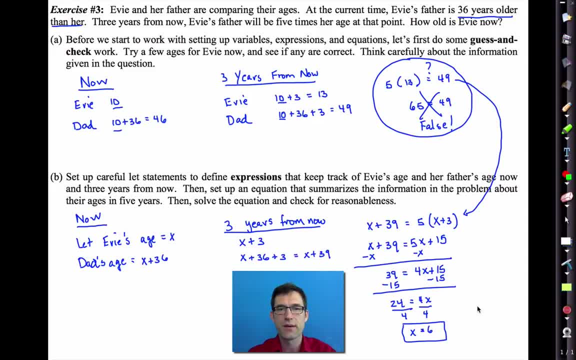 I'm doing to the variable X. Okay, Certainly seems reasonable. Just for a moment, talk about some things that wouldn't be reasonable. Number one: it wouldn't be reasonable if Evie's age came out to be negative. Number two: it wouldn't be reasonable if Evie's age came out to be negative. 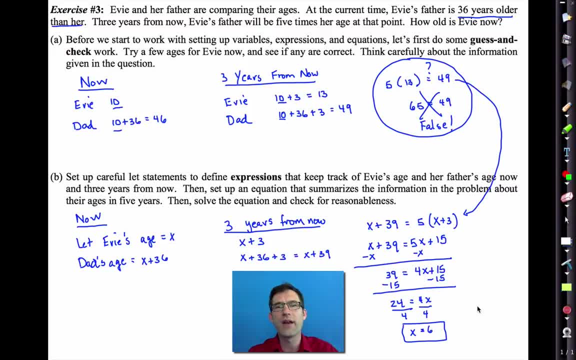 Number three: it wouldn't be reasonable if Evie's age came out to be negative. Number four: it wouldn't be reasonable if Evie's age even turned out to be a non-integer fraction, like if I had gotten 6.3.. 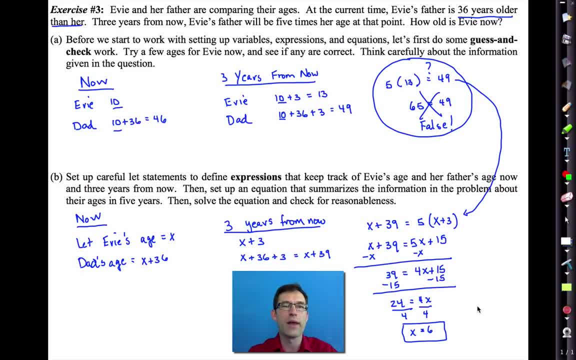 We don't report ages that way, right? When you ask me what my age is, you know I'll say that my age is 43, let's say, Okay, I won't say that I'm 43.8.. Of course, some kids talk about their ages in terms of halves. 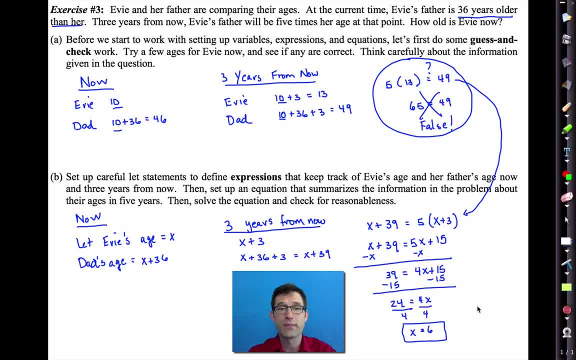 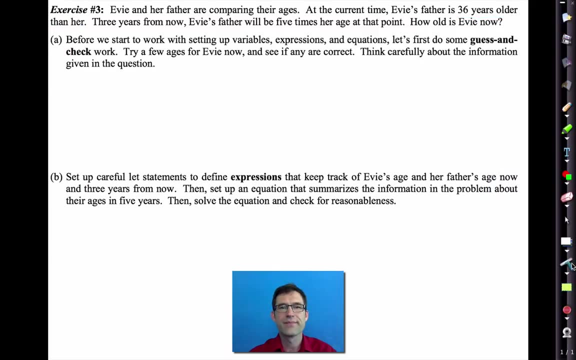 But generally speaking, we report ages in whole numbers. Okay, So pause the video now If you need to copy down what you need and then I'm going to scrub out the text. Okay, Here we go. Let's move on. 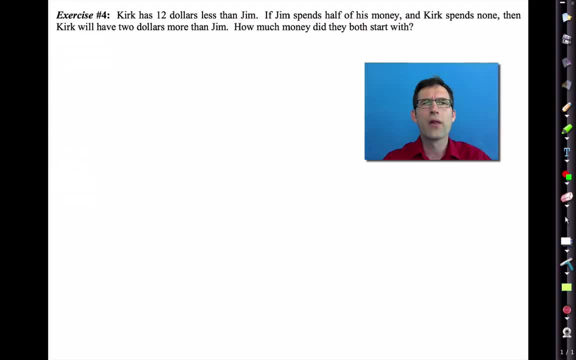 Okay, Exercise four: Kirk has $12 less than Jim. If Jim spends half of his money and Kirk spends none, then Kirk will have $2 more than Jim. How much money did they both start? Let's start with Wow, Okay. 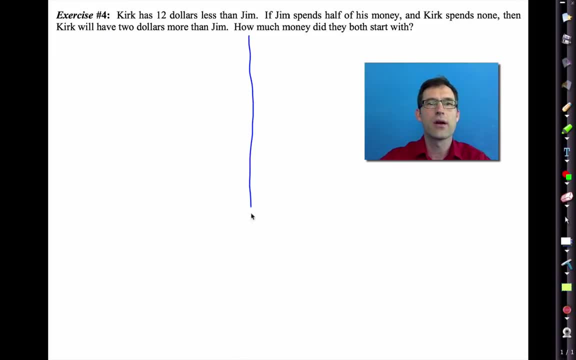 Well, again, let's do a little guess and check over here. right, Guess and check over here, and then we'll play around with the algebra over here. So notice that Kirk's money is based on Jim's money. That's actually kind of important in how we attack this problem. 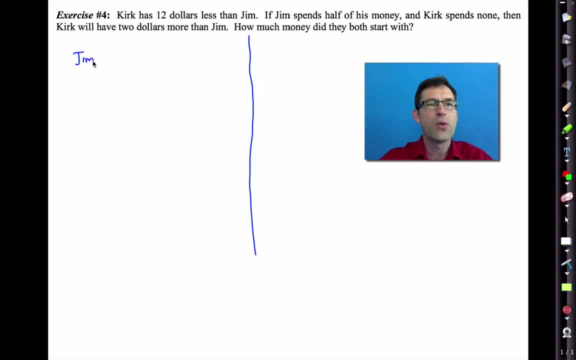 Kirk has $12 less than Jim, So why don't we start off with Jim having, let's say that Jim has $50.. Okay, Then of course, Kirk will have $50 minus $12, which will equal $38.. 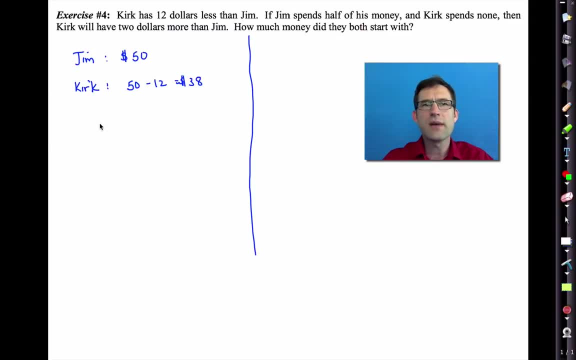 All right, Then if Jim spends half his money, right, So after we spend money, right, Jim has one half of $50, which is $25.. Then Kirk will have two more dollars than Jim. Well, Kirk has $38 right now, right. 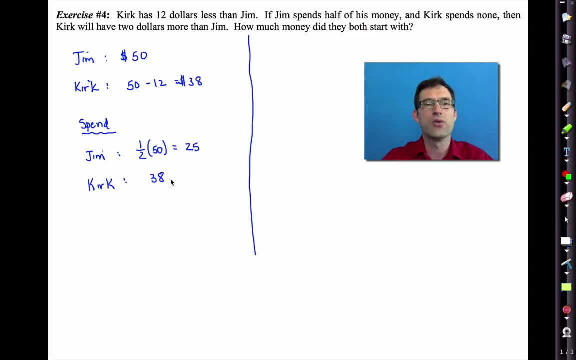 And specifically, Kirk is supposed to have $2 more than Jim. In other words, if I take $2 and I add it to Jim's money, right, Then I should get Kirk's money. but 38 doesn't equal 27,, right? 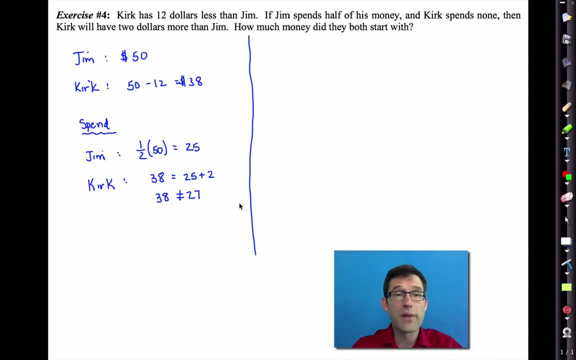 So Jim didn't start with $50.. That's all that tells us. Okay, But watch as we manipulate. So let's let M be equal to the amount of money Mummy- Hopefully no mummies today- The amount of money Jim has. 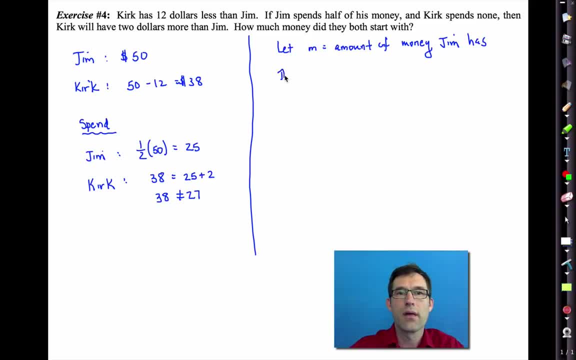 All right, Kirk, Then M minus $2.. M minus $2 equals the amount Kirk has. All right, Fair enough, right? Then after they spend money, because that was originally, Jim now has one half M and Kirk still has M minus $12.. 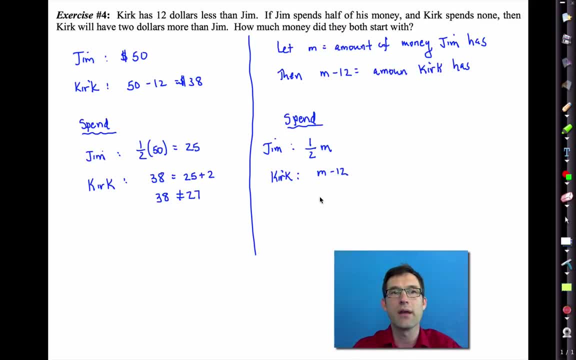 Now, what does it say, though? It says that if Jim spends half his money, Kirk will have $2 more than Jim. This is the hardest part, right? Kirk's amount of money, which is M minus 12, will be Jim's amount of money, which is one half M plus another two, right? 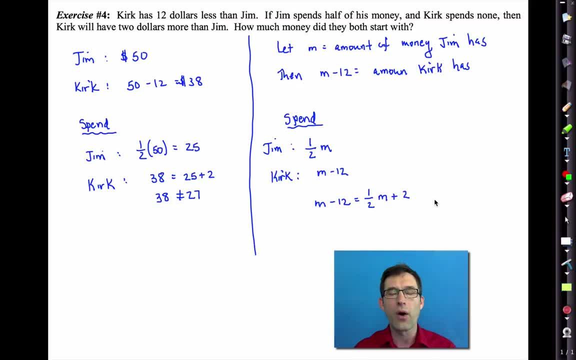 And that's tricky because it would be very understandable to think, oh, I'm supposed to take Kirk's money and add two to it to get Jim's money, But then that would mean that Jim has two more dollars than Kirk. But Kirk, right, which is M minus 12, has two more than Jim. 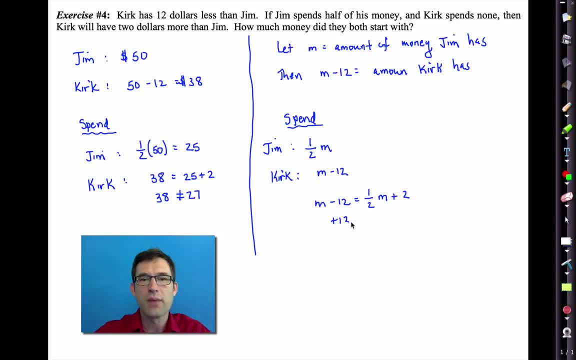 All right, Let's do some solving. We're good to go right. So I'm going to use the additive property of equality to add 12 to both sides. I'll have M equals one half M plus 14.. I'll use the additive property of equality to subtract one half M from both sides. 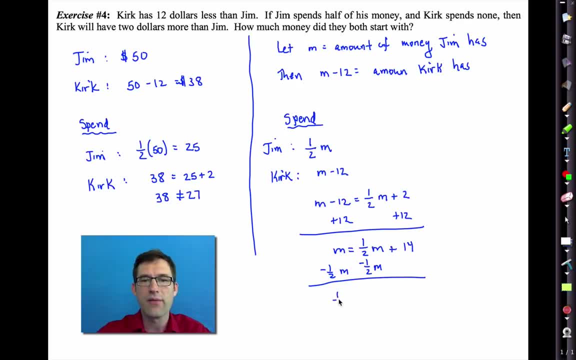 Don't get scared about fractions: One M minus one half M will be one half M, That'll be 14.. And now I can use the multiplicative property of equality to multiply both sides by two to find out that Jim had $28.. 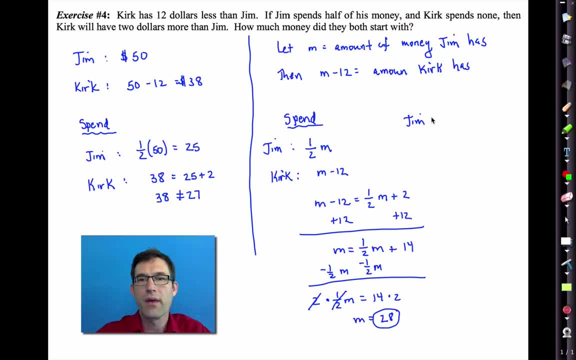 So Jim originally had $28 and Kirk had 12 less than that, so 16.. Now what's interesting is that this one's a real easy one to solve. We're going to check- Watch as we check- for reasonableness, right. 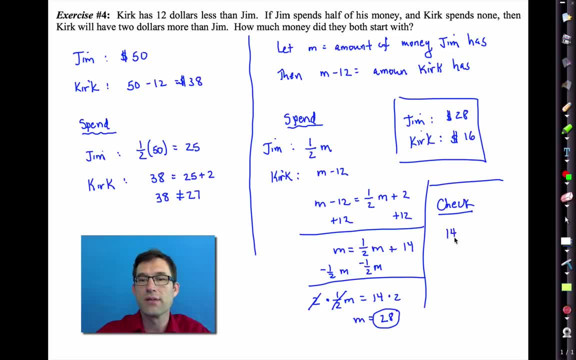 Because what did it say? It said: when Jim spent half his money, right, so Jim has $14 left. Kirk will have $2 more than Jim. Well, Kirk has $16 and notice that that is two more than what Jim has. 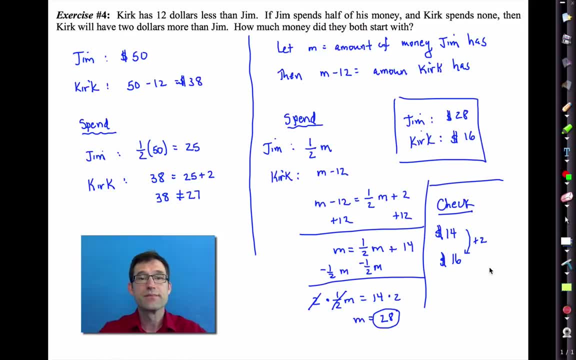 So it makes sense, given what we were told in the problem. All right, I'm going to clear out that text. Think about, Think hard about what we did with the example and then how we translated that into the algebra. All right, 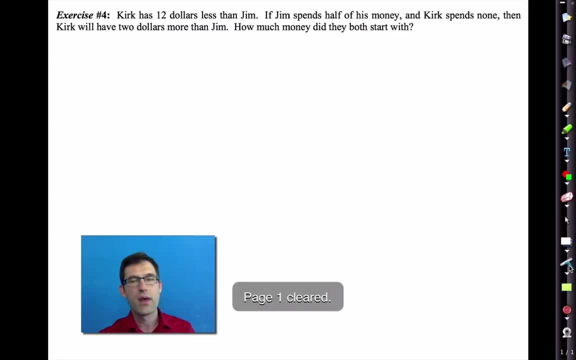 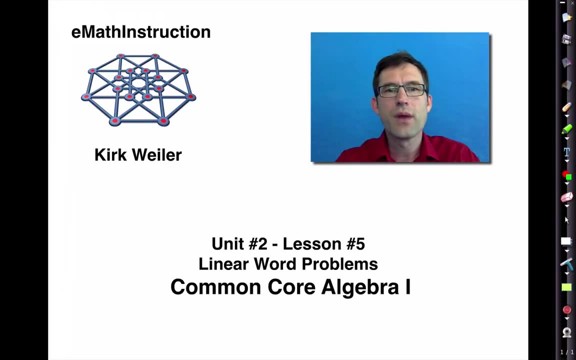 Here goes the text. Clear it up. All right, Let's wrap it up. So we did some modeling today. We took some real-life scenarios, We tested them with just numerical values. Then we used that process to develop equations that modeled the scenario and then solved. 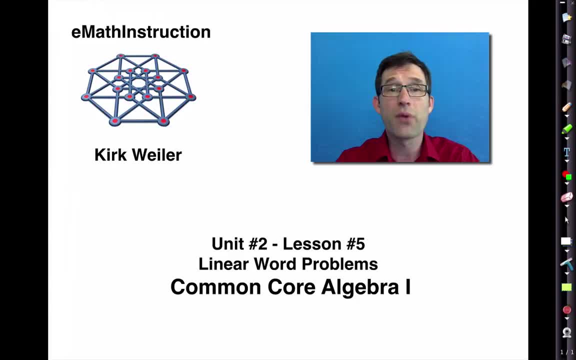 those equations to find out what we wanted. This is a tough process- It really is, because it combines equation solving techniques along with translating English into math, and that can be a struggle for students. I guarantee, though, that if you stick with it, if you keep working at it, you will be.